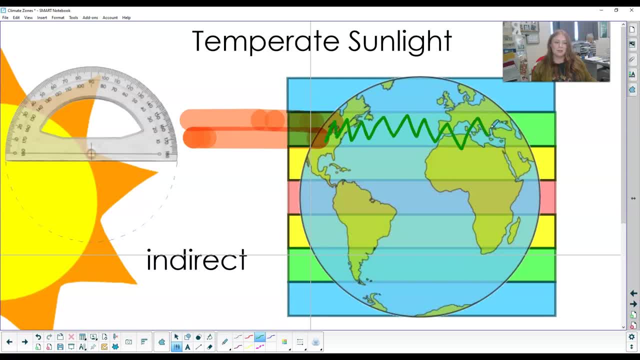 and then we are up here, so above the form, below the poles, and our sunlight hits us here, So you can see right, we're more at an angle now, So we're starting to get that indirect sunlight. So now we're to a hundred and about 37 degrees. So we went from 120 before, now we're to 137. 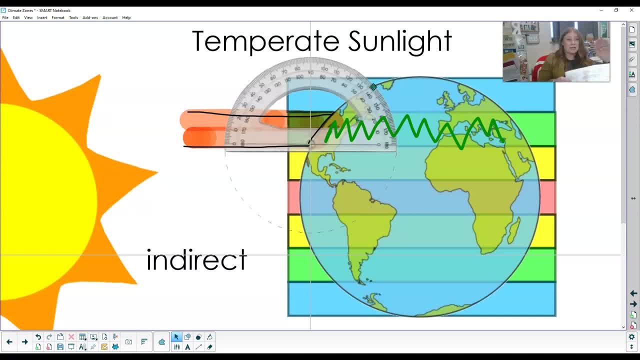 So we're at a hundred and thirty-seven degrees. So now we're at a hundred and thirty-seven. So now we're to a hundred and thirty-seven. So we went from 120 before. now we're to 137.. So you can see, right, we're angling even more. That light's really having to spread. 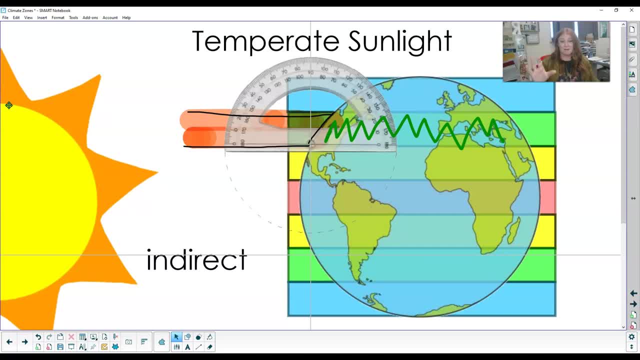 more to reach us. So it's getting the same amount of light. that same band is coming toward us, but it's having to spread to cover that area more. So that's why we get those different seasons is because when we're tilted toward the sun, we'll get summer. 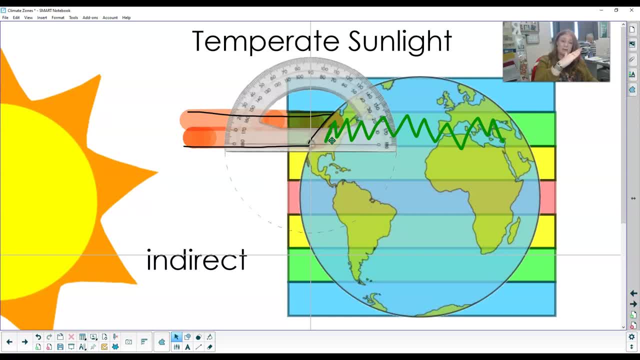 When we're tilted away from the sun, we will get winter, And then in spring and fall it's just like the sun is here, it's just getting the equator and the poles are just getting equal amounts of light, So most of the sun is hitting at the equator. 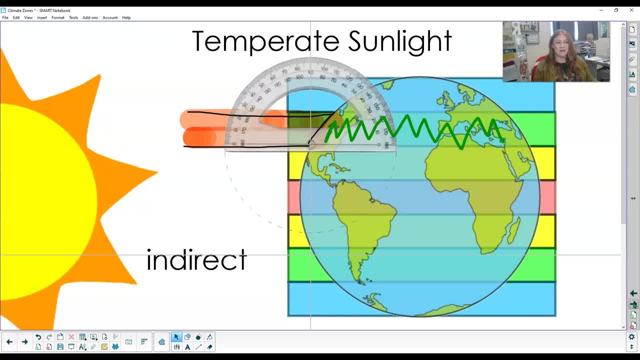 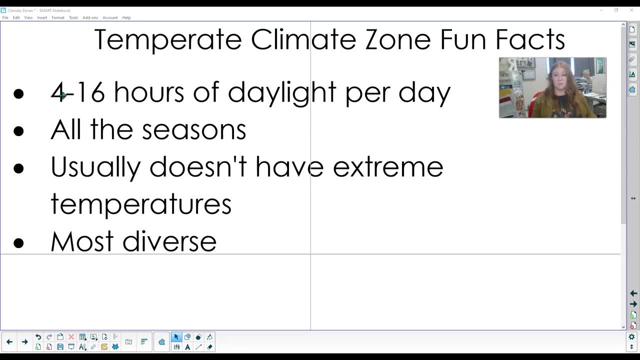 Okay, fun facts about temperate climate zones. So we can have anywhere from 14 to 16 hours of sunlight per day. So four is pretty crazy. That's going to be pretty far north or south toward those poles. So right if they're tipping. if I hadn't tipped away from the sun I wouldn't have. 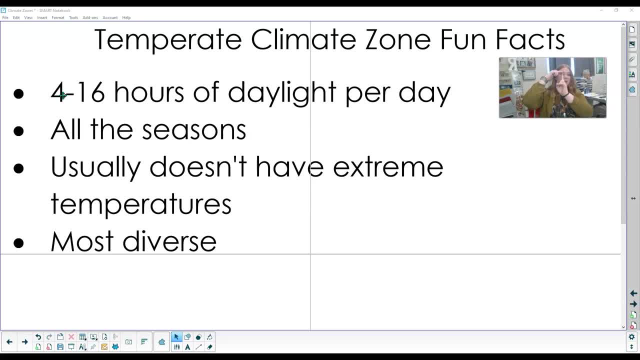 tipped away from the sun, I'm not going to get very much sunlight during my winter time. So, like if you live in Alaska, they during the winter they get very little sunlight because they're so far north and we're tipped away from the sun and we just they don't get. 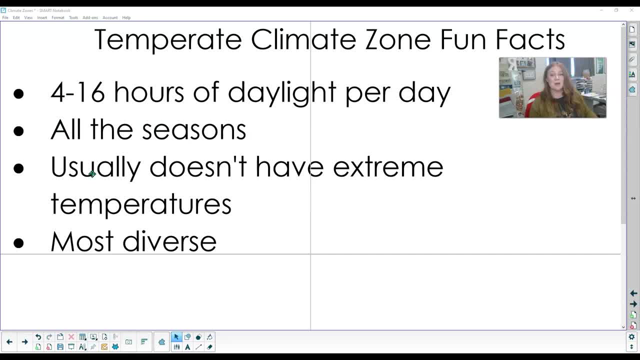 that much sun- Kind of crazy. So we have all four seasons. We usually don't have super extreme temperatures. Like we're not going to have temperatures that are 130 degrees in the summer, We're also not going to have temperatures that are 130 degrees in the summer. We're also not going to 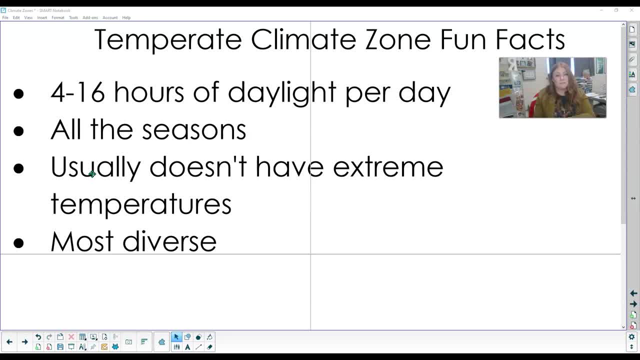 get you know, down into like 40 degrees negative and it can happen. but we don't have like crazy, crazy highs and lows. We just we get hot in the summer, we get cold in the winter.